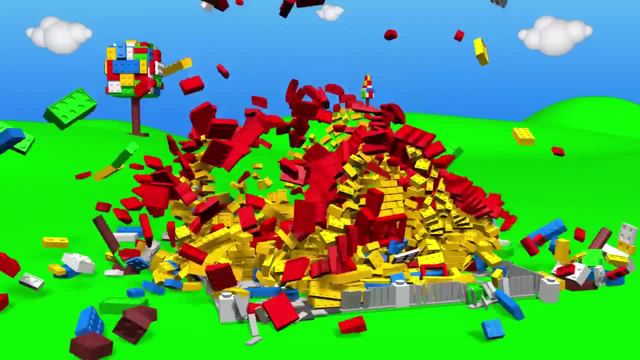 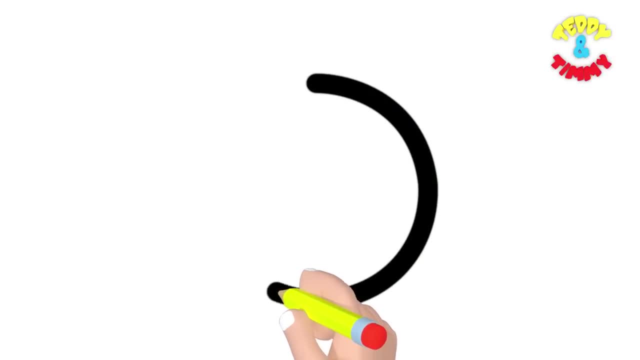 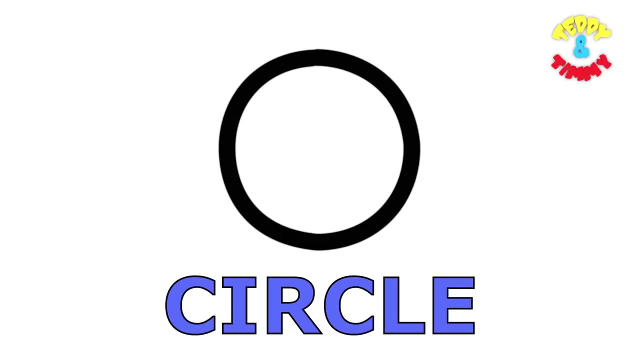 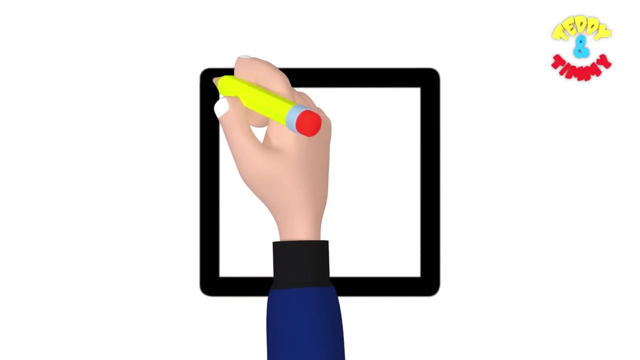 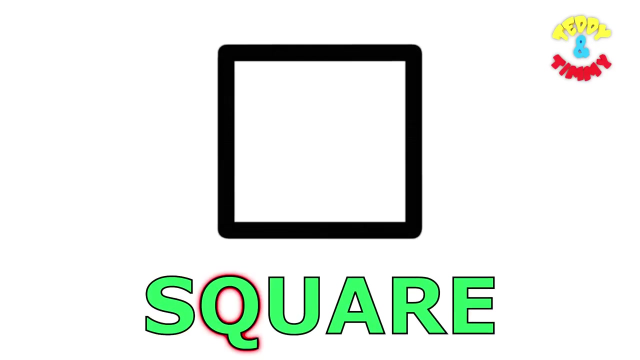 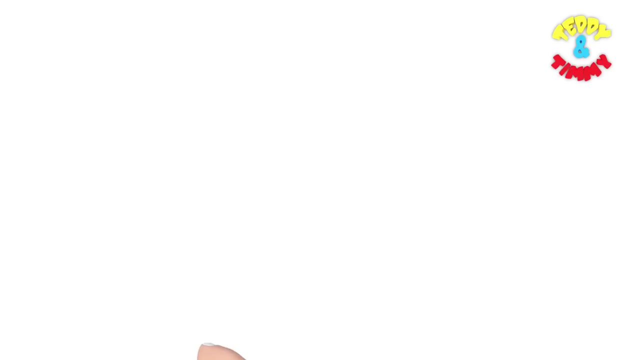 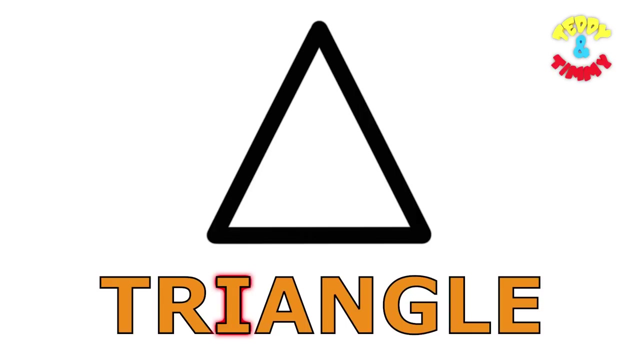 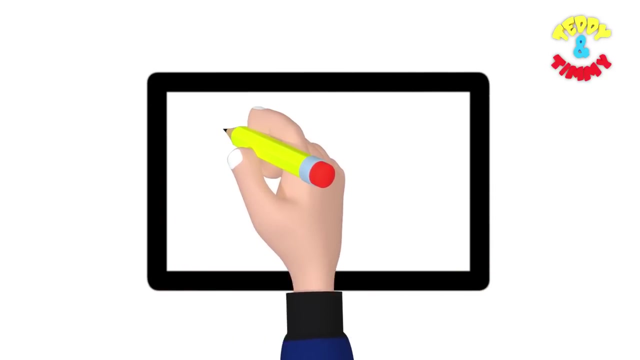 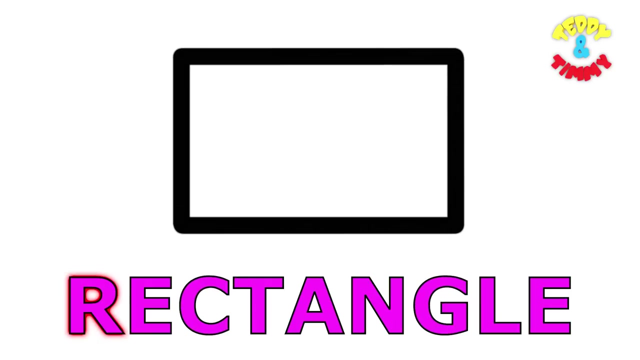 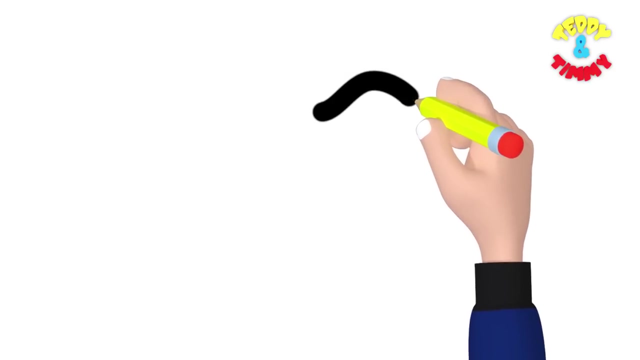 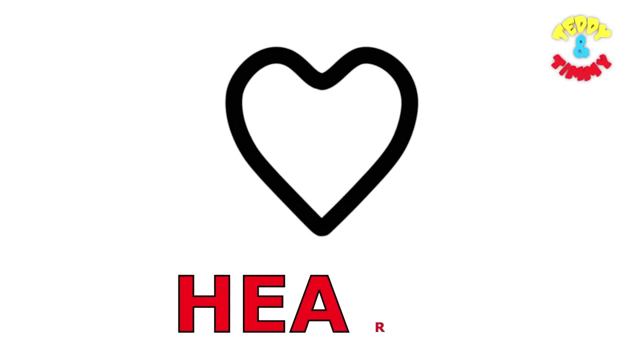 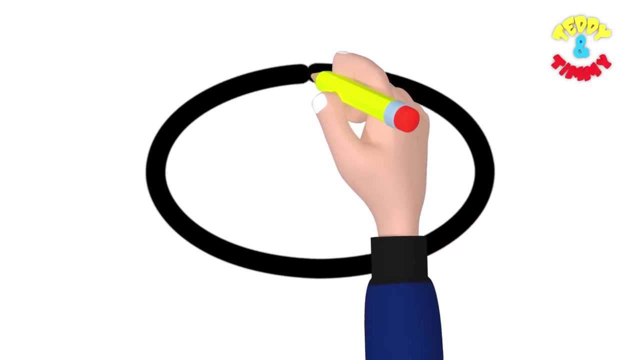 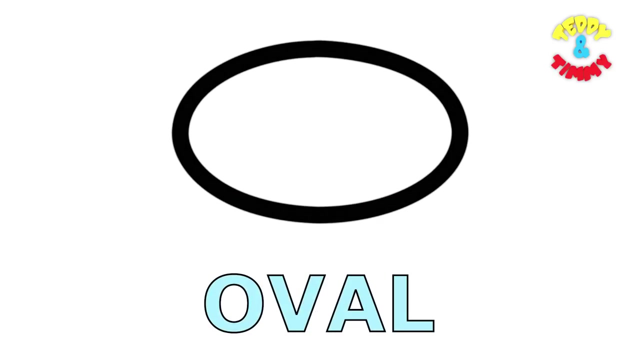 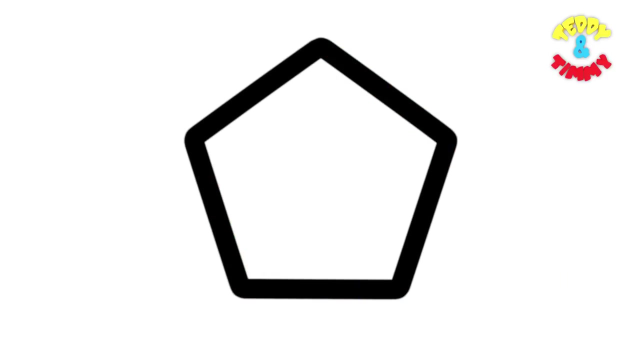 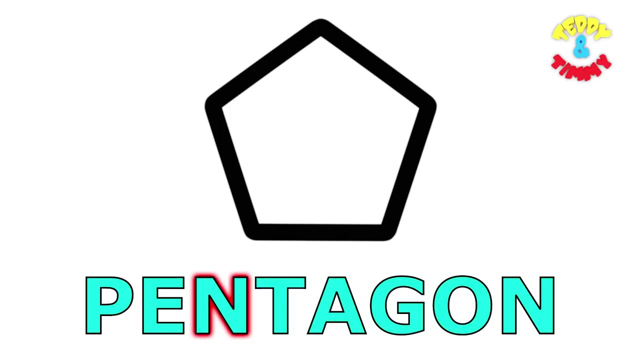 Circle C-I-R-C-L-E Circle Square S-Q-U-A-R-E Square Triangle Triangle- T-R-I A-N-G-L-E Triangle Rectangle- R-E-C-T-A-N-G-L-E Rectangle- Heart- H-E-A-R-T. Heart Oval S-O-V-A-N-G-O-N-T-A-G-O-N-T-A-G-O-N-T-A-G-O-N-T-A-G-O-N-T-A-G-O-N-T-A-G-O-N-T-A-G-O-N-T-A-G-O-N-T-A-G-O-N-T-A-G-O-N-T-A-G-O-N-T-A-G-O-N-T-A-G-O-N-T-A-G-O-N-T-A-G-O-N-T-A-G-O-N-T-A-G-O-N-T-A-G-O-N-T-A-G-O-N-T-A-G-O-N-T-A-G-O.